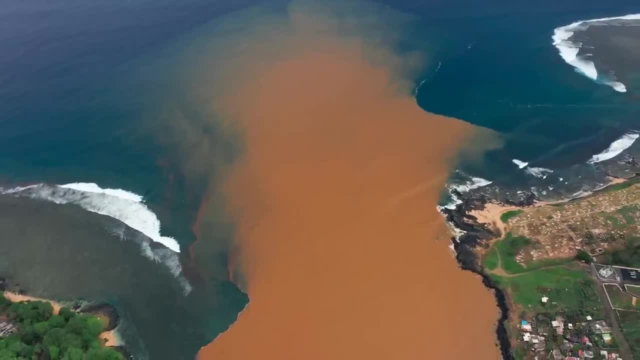 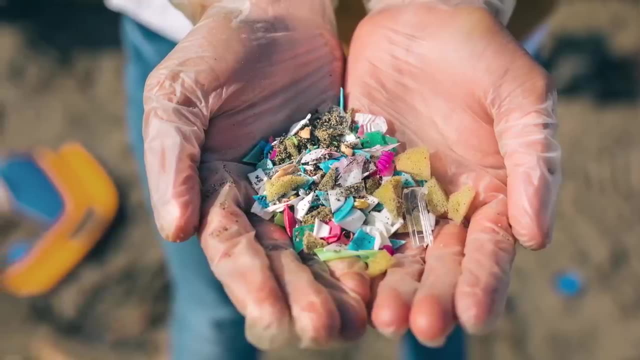 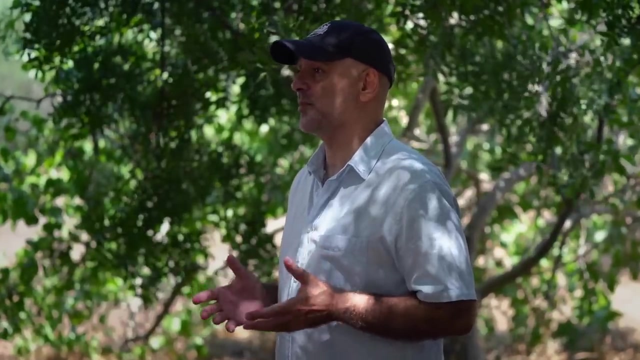 rain Rivers are being heavily polluted by agricultural chemicals, creating huge dead zones in our oceans, which are full of microplastics, as is the air that we breathe. The list goes on, and it is so easy to feel desperate and overwhelmed about all of this, but I believe there is hope for the survival of 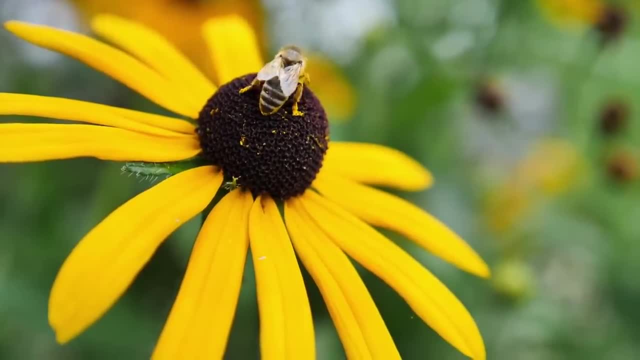 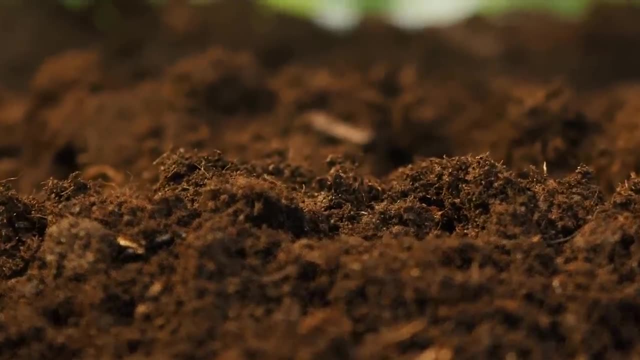 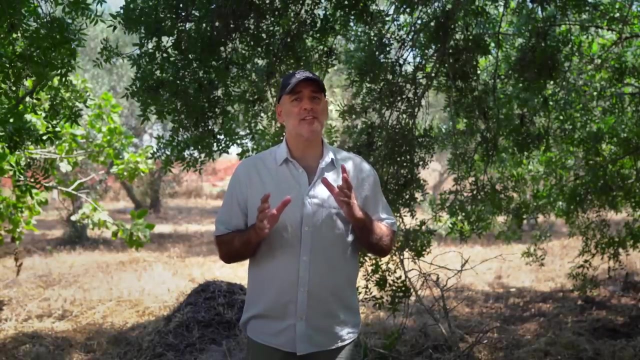 our species and for the other life forms with which we share the planet. Many of the biggest problems we face are connected to the way we interact with the earth's soil and to the way we farm. This is our focus at the Soil Food Web School In 2015,, while taking some time out. 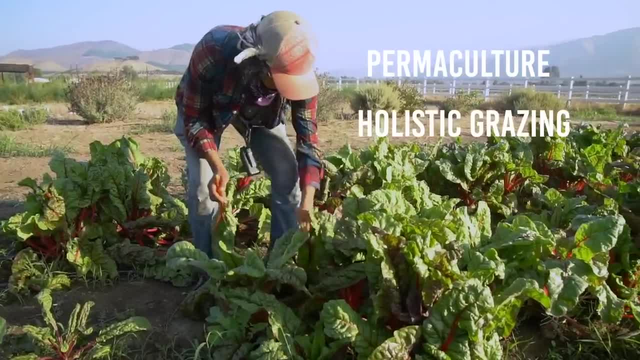 I came across the world of permaculture and holistic grazing, soil biology and regenerative agriculture. I was so excited to be part of the Soil Food Web School and to be part of the Soil Food Web School. I was so excited to be part of the Soil Food Web School and to be part of the. 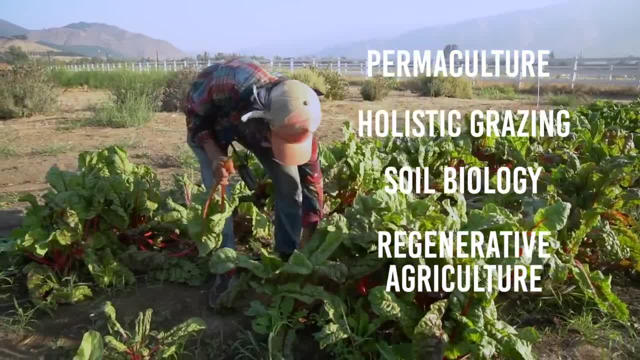 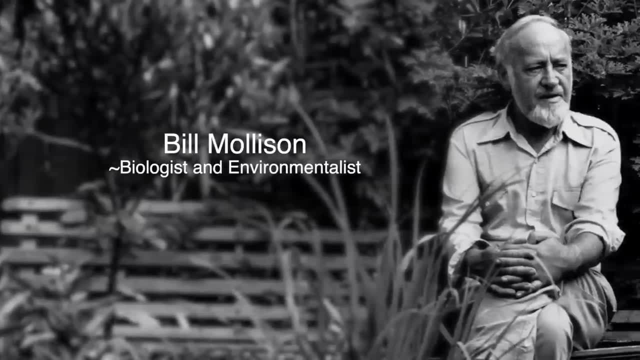 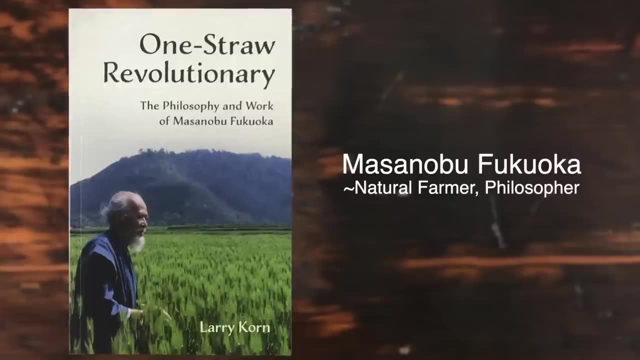 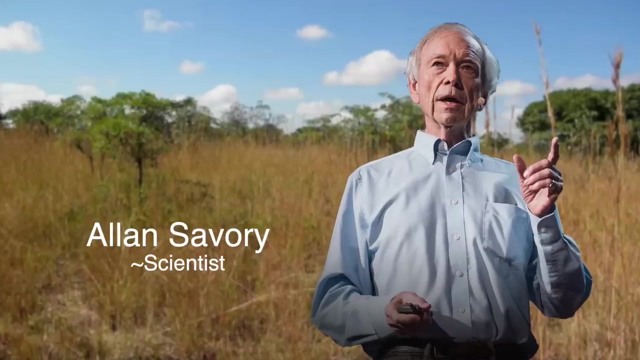 agriculture and I began to realize that there are real, tangible solutions to many of the existential threats we face today. I learned about farmers and scientists who had been experimenting with new techniques that can be used to support nature's recovery. Some of these people had found ways to increase yields and profits without using any harmful chemicals, and 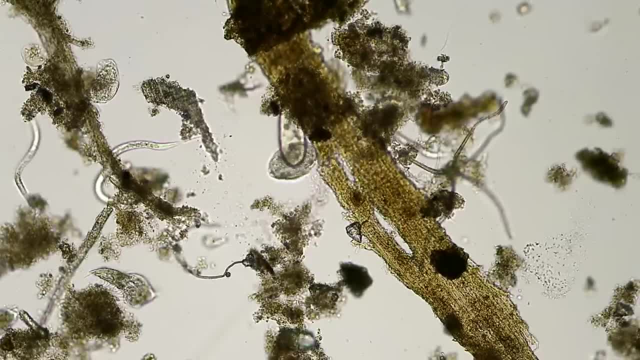 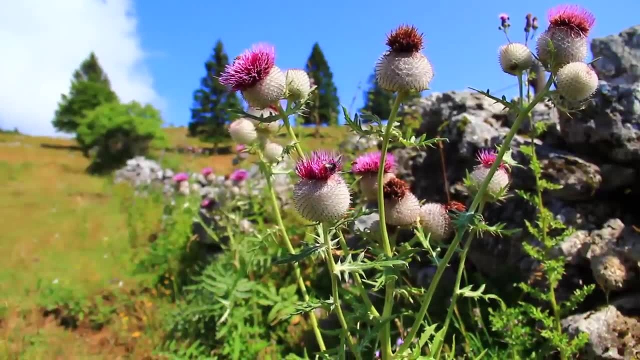 without plowing the land. I learned about the members of the Soil Food Food Network and its partners who are working to study how to reduce the risks of carbon emissions. They tend to tackle these problems first hand, which causes huge damage to the microscopic world within the soil. These methods promote the 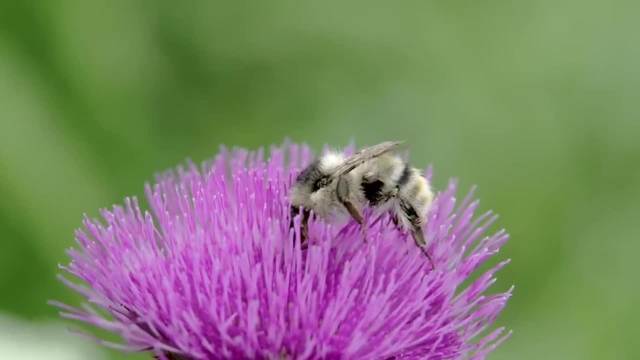 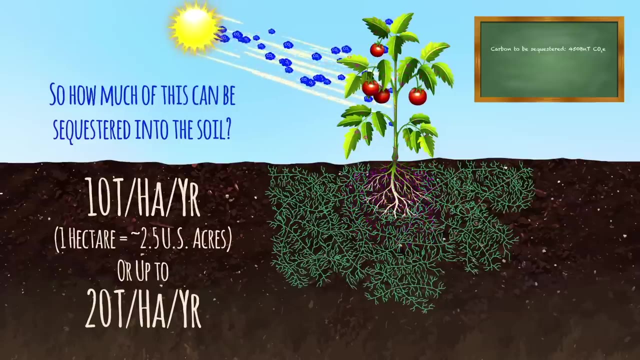 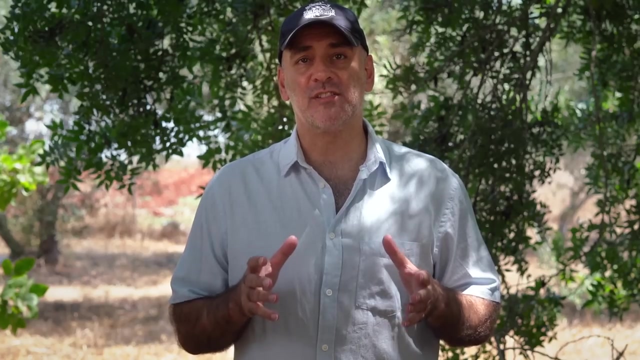 recovery of natural systems, and they have a regenerative effect on the wider ecosystem. I also learned that the soil has the potential to absorb many billions of tonnes of atmospheric carbon and to lock it away for hundreds and even thousands of years. This gave me real hope and I realized. 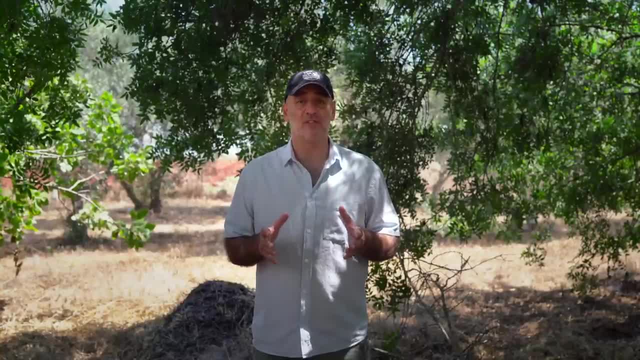 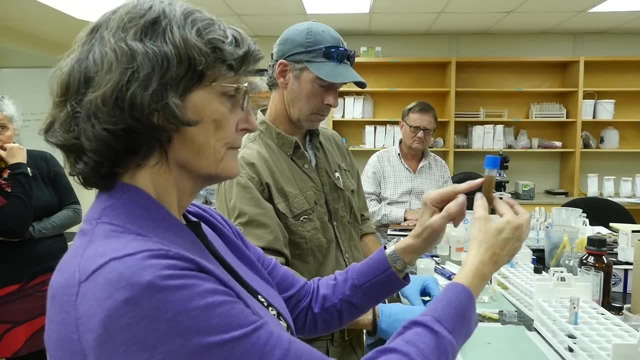 and so I decided to dedicate the rest of my life to this course. Over the last three and a half years, I've been honored to work with Dr Elaine Ingham to help make her invaluable teachings available to the world through the Soil Food Web. 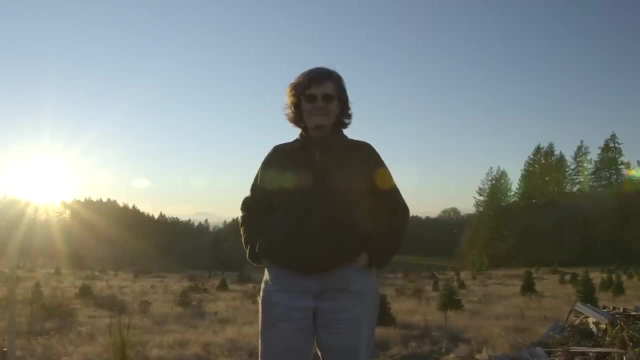 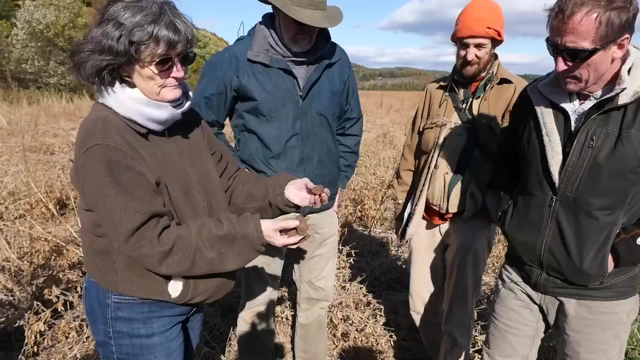 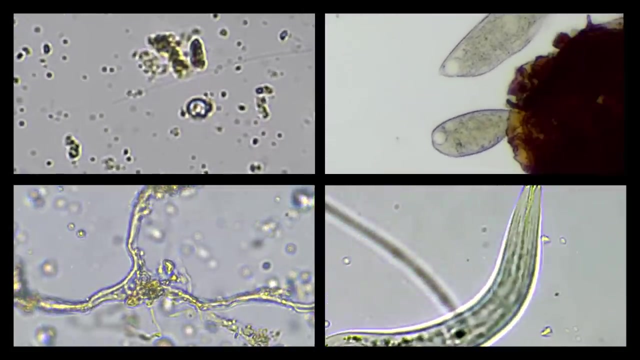 School. Dr Elaine is one of the most renowned soil biologists in the world. In the 80s and 90s, she and her colleagues pioneered research in soil biology, documenting the four key groups of beneficial microorganisms that are required to make a soil functional. Over the last four decades she's worked with 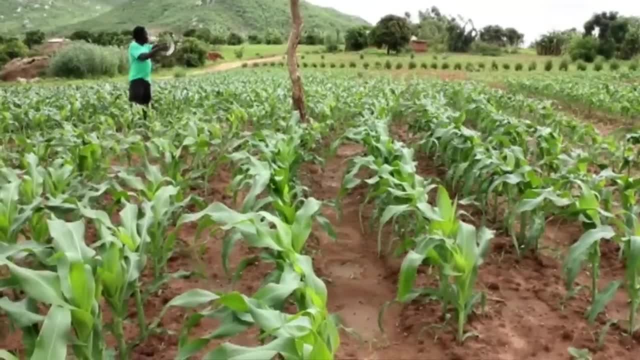 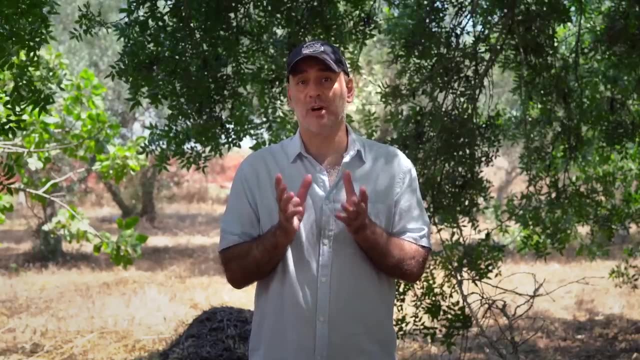 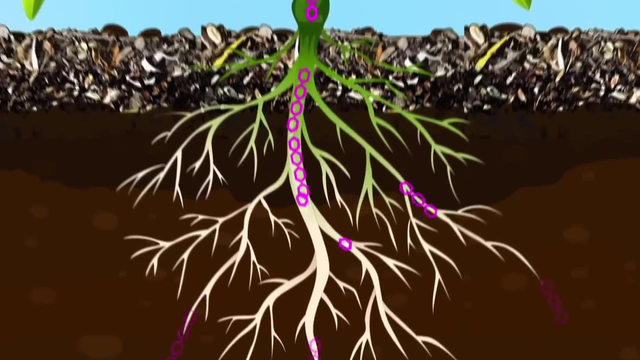 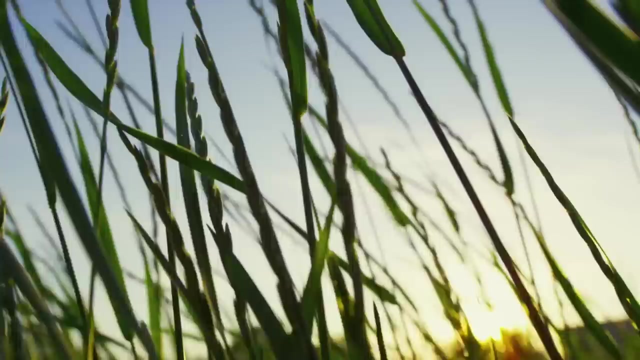 farmers on six continents to develop the Soil Food Web approach: a scientific and holistic way of rapidly restoring that soil biome to a healthy level. Once restored, soil biology forms a symbiotic relationship with plants and crops and nourishing and protecting them without the need for chemical inputs. This is 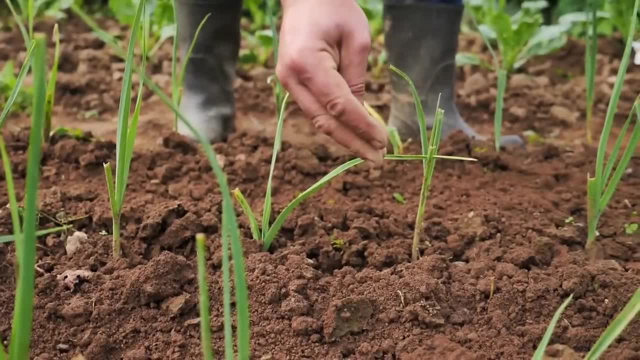 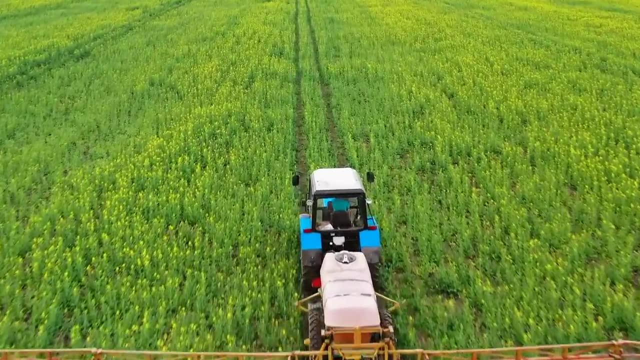 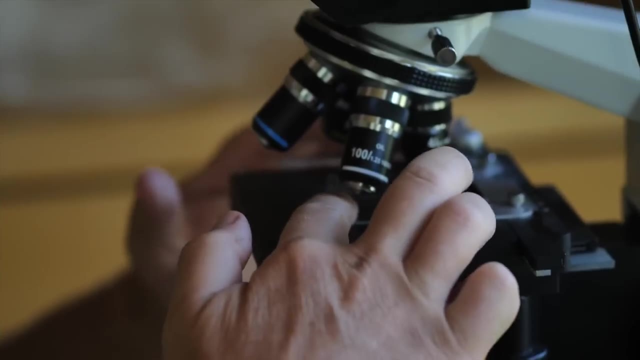 what nature has been doing since the beginning. Farmers who adopt this approach can liberate themselves from the need to use expensive fertilizers, herbicides and pesticides, reducing their costs dramatically without harming their profits. Since 2019, the Soil Food Web School has been providing training. 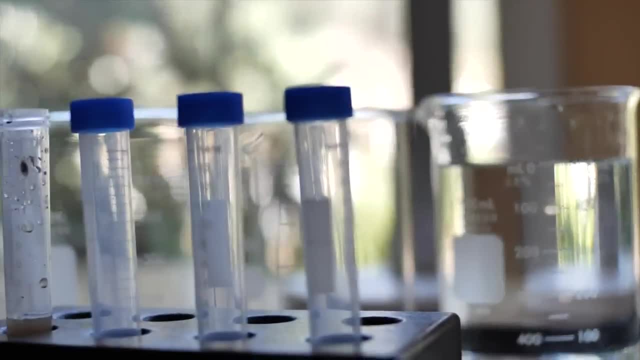 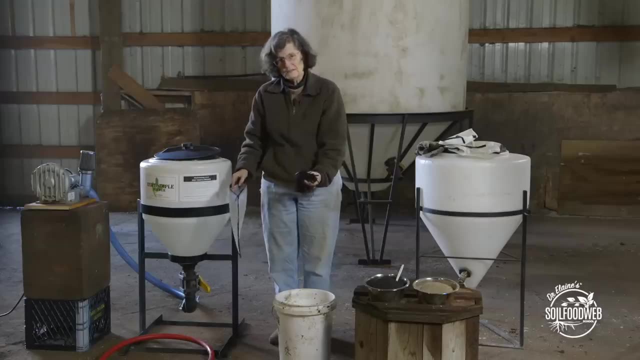 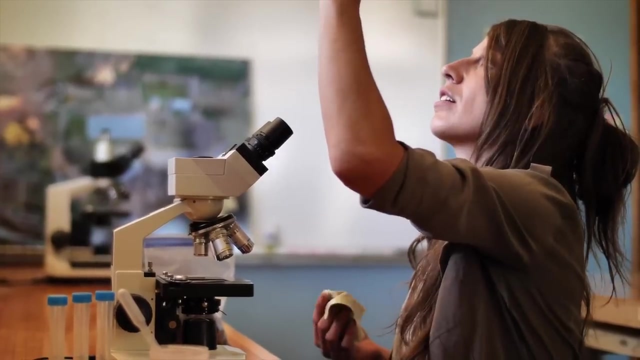 to individuals and organizations around the world, Empowering them to rapidly regenerate the soils in their communities using Dr Elaine's methods. Some of our students are farmers or agronomists, and some have no industry background whatsoever. They're ordinary people who want to make. 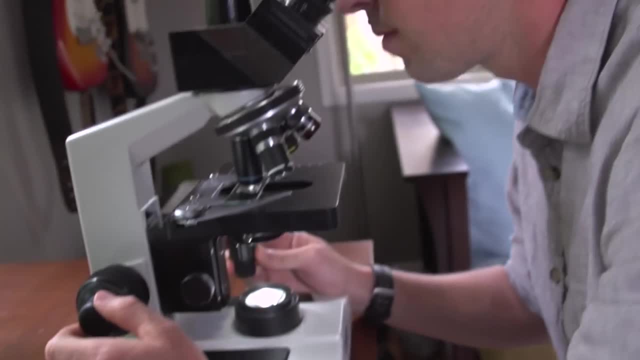 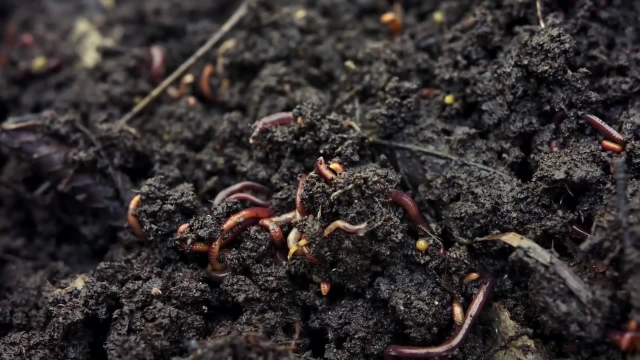 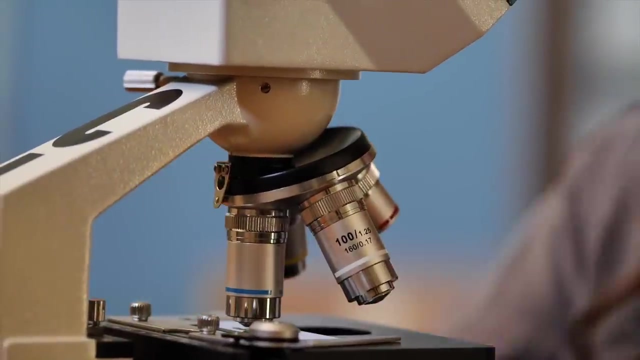 an impact. They can do this by obtaining the skills required to support farmers in making the transition to regenerative agriculture using the Soil Food Web approach. Anyone can make an impact. In some of the other videos on this page, you'll meet folks who have transformed their lives by becoming Soil Food Web consultants. 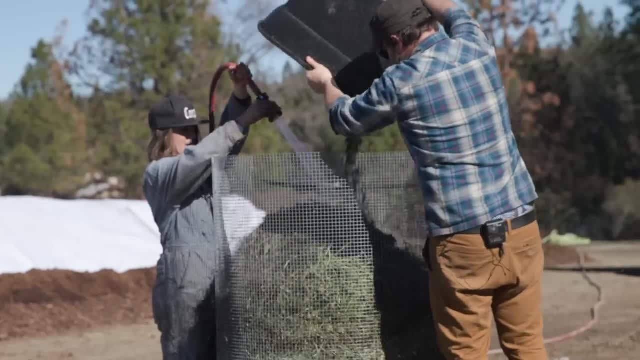 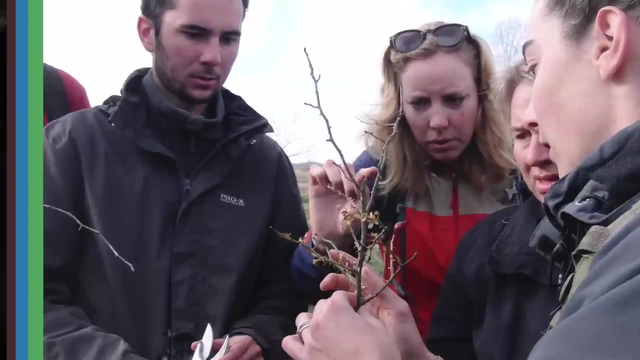 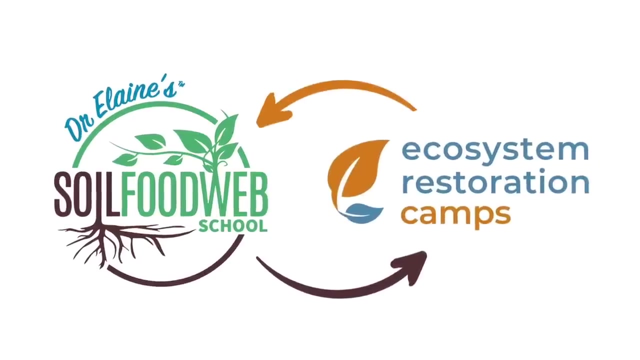 lab technicians or compost producers. Many of them are now running successful businesses and are feeling great about the contribution that they're making. Today, the Soil Food Web School is entering a new chapter. We're deeply honored to be partnering with Ecosystem Restoration Camps to develop a 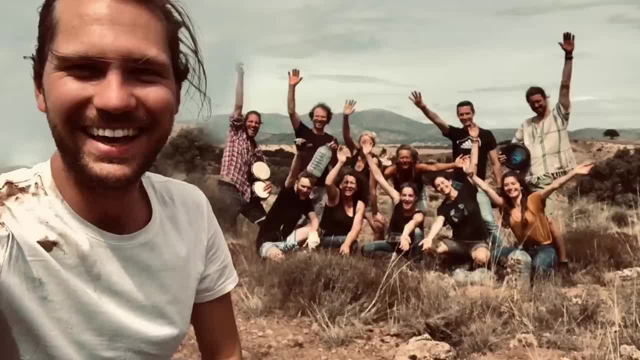 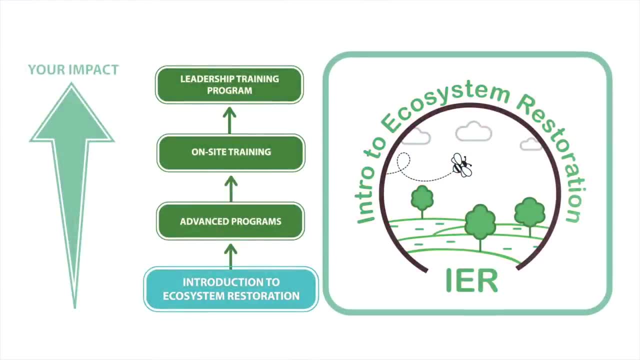 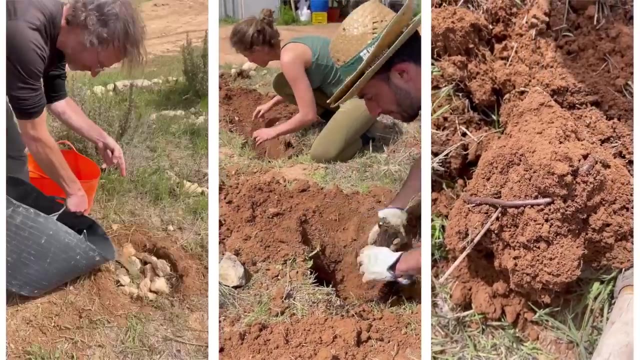 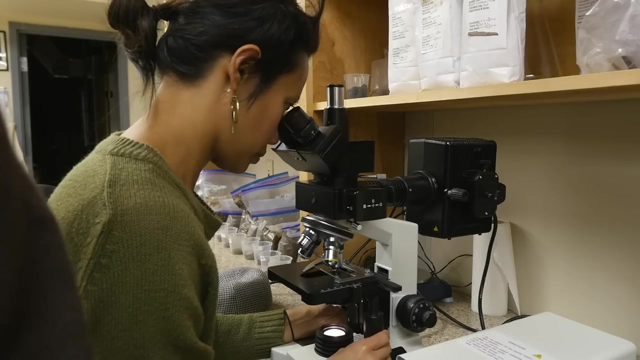 series of new courses designed to help our students make an even bigger impact. The introduction to Ecosystem Restoration is the first of these courses, and it is designed to give our students a better understanding of ecological principles and how ecosystems can be restored at scale. Together with the Soil Food Web approach, this is a powerful combination that will 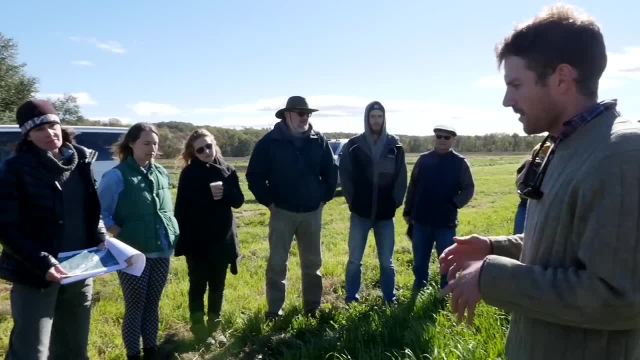 maximize the impact our graduates can have on the earth. We're in Cranston, New York, today and a Cranston school that is a family of soil upcoming this spring. We're in Cranston, New York, today and a Cranston school that is a family of soil upcoming this spring.